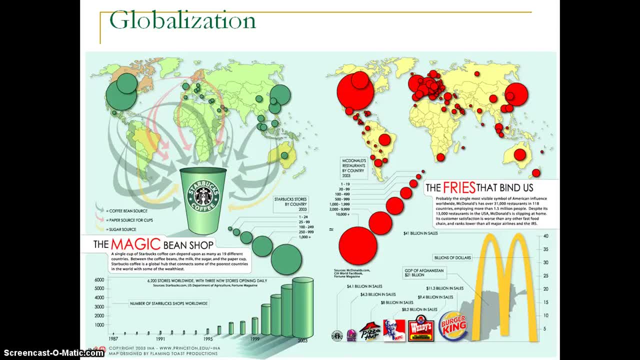 in another kind of way, and this is, of course, again talking about economic globalization. but really, I see, when we look at the graphic or the map over here of Starbucks and McDonald's, I really see two different examples of globalization taking kind of being illustrated here. Well, first we look at Starbucks and if you'll notice the map here, you can actually say this is both a choropleth map. you could also talk about it being a proportional symbol map, and we'll talk more about that as we get into the to the unit. but you see here, really the idea here is that 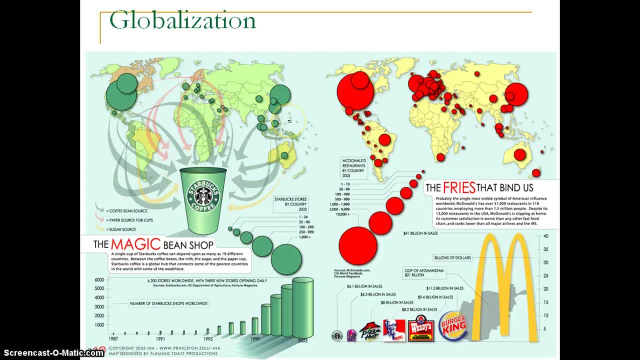 is that Starbucks is reaching around the world to collect products for its coffee. So when you go to Starbucks in the morning, I know a lot of my students go to Starbucks and they don't get coffee. they get some kind of frozen latte to pretend like they're drinking coffee. 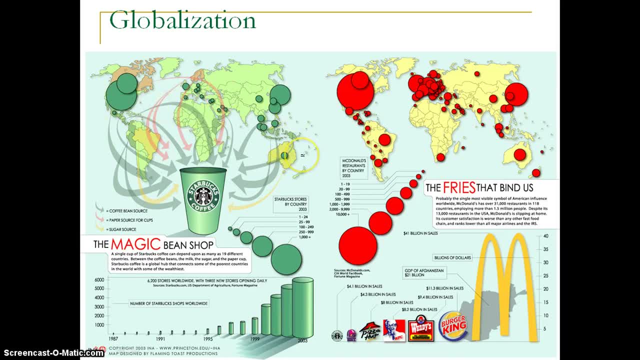 and feeling sophisticated. But if you look at this, you see they reach around the world to get their products. whether it's the coffee beans, they may be coming from South America, maybe Africa, or they're talking about the sugar products, which may be come from Brazil. 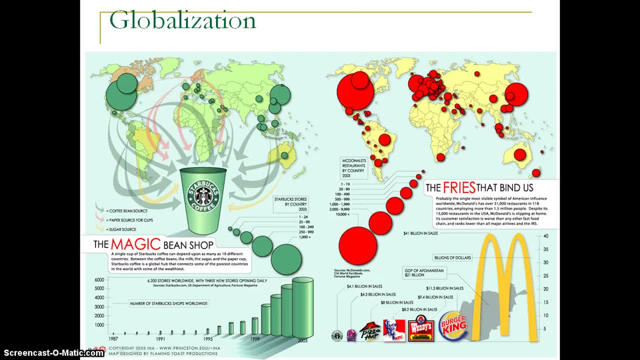 and you see also they're illustrated Australia, or the paper products for their cups and things along those lines, And so that's really what's being illustrated here in this idea of globalization, bringing companies able to reach across the world to bring products together for sale in a location. 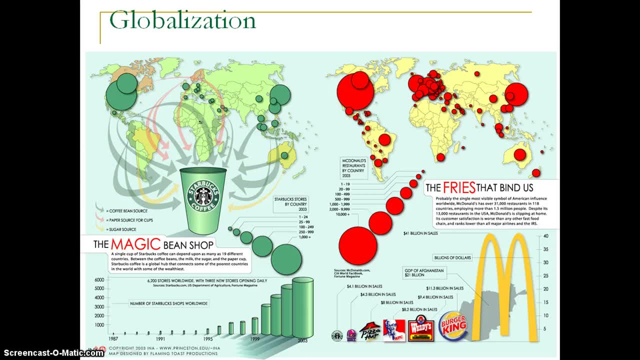 And you think about how that is only possible because of our modern transportation system. But then also you think about modern economics, because you look at a cup of coffee at Starbucks and it costs a couple of dollars, maybe $2 or $1.50, I forget what the exact price is. 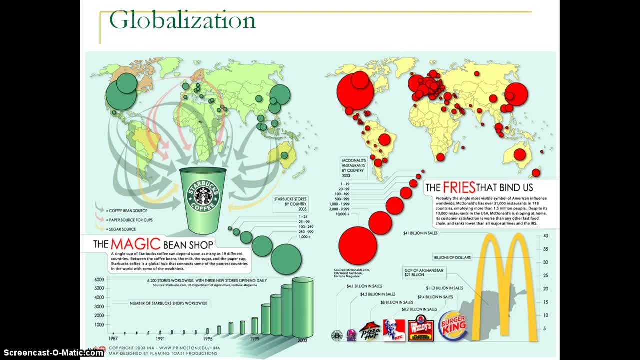 of a Starbucks cup and that's just a regular cup of coffee. That can be a tremendous expense to a lot of people around the world, but when you talk about a very large middle class that is able to have disposable income enough to buy on a regular basis a $2 to $3 to $4 coffee drink, 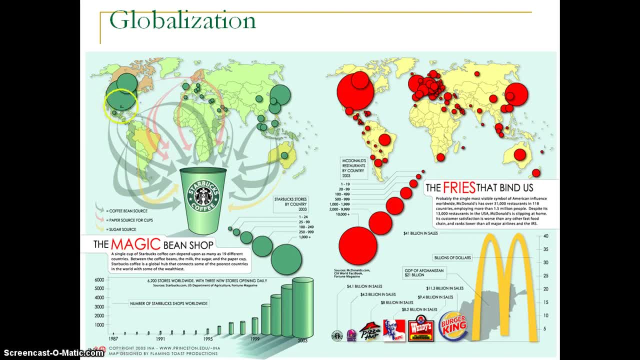 that says a lot about the local economy, And so this, of course, you could also talk about the way that it employs people around the world through the purchase of products at a Starbucks. Okay, so we look at economics and the way that Starbucks has reached across the world. 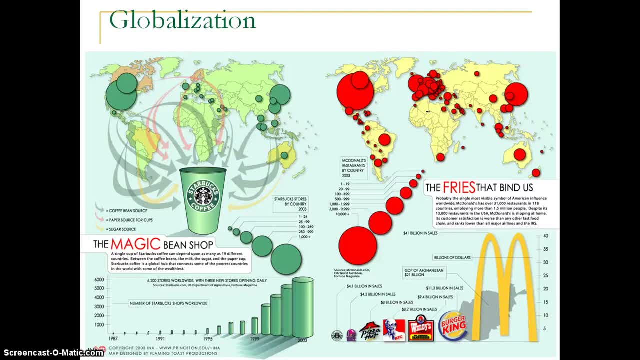 to get all their products. And then we move here to the graphic of McDonald's, and this is talking about the number of McDonald's restaurants in a country, And so you see the way that Western companies have spread themselves across the world and you have this company. 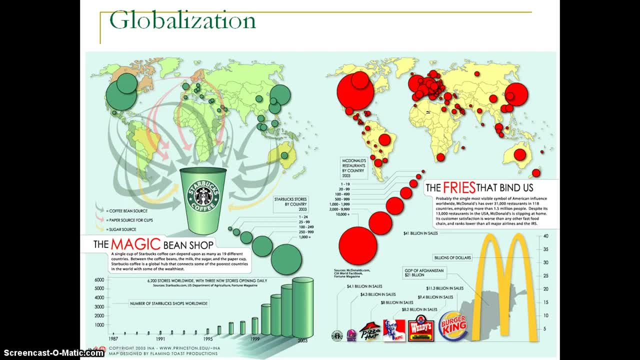 that is able to sell its product all across the world. Now, one of the interesting things about a McDonald's is that it actually will adapt its menu based upon the country that it is in. You know, you look at places like India, where you have predominantly Hindu population. 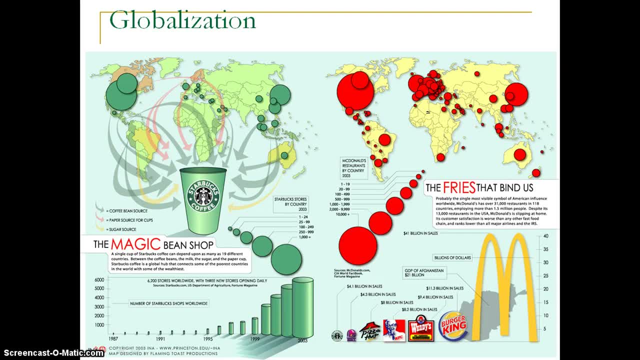 that is not going to be eating beef products, And so there's a lot of vegetarian options, There's a lot of options that are gonna be more sensible to their religious convictions and things like that. Same thing with some of the Arab countries. We have predominant Muslims. 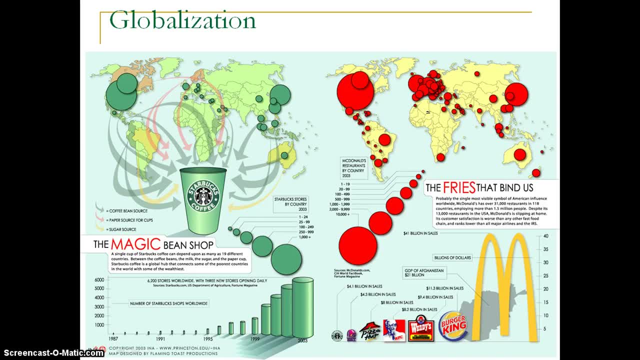 You're not gonna have any pork products And so they're gonna shy away from those things. And you also have some interesting things, like in Thailand. they have these little shaker bags where you take a seasoning, you pour it over the fries and shake it. 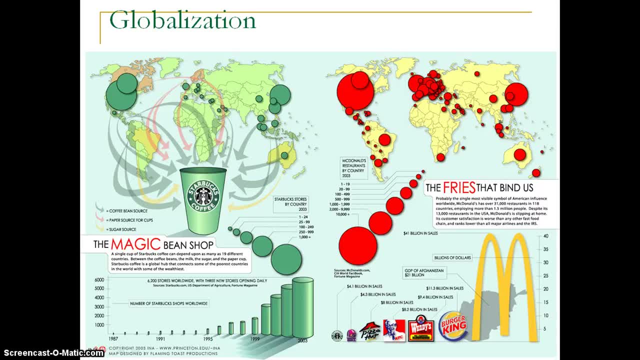 and apparently that's a favorite treat for them, a favorite item for them. So the actual McDonald's restaurant is spread across the world, but they're actually going to be changing their menu as they go from country to country. So you look at globalization in that way. 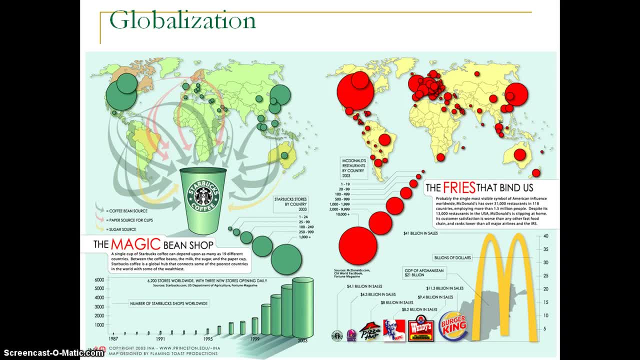 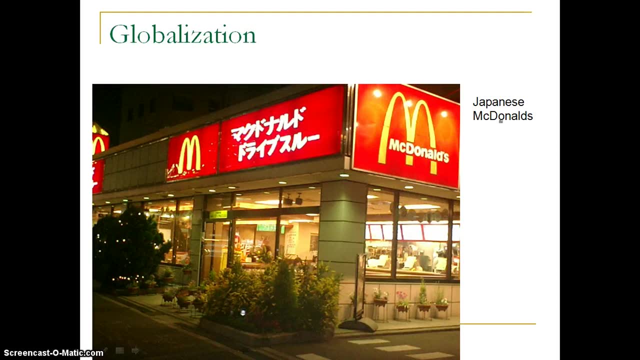 And again, I see these two graphics as two different elements of globalization in terms of economics. And then, of course, this is just an example of a McDonald's that's in Japan. Now, one of the elements of globalization that you notice is that now, of course, there's the giant arches. 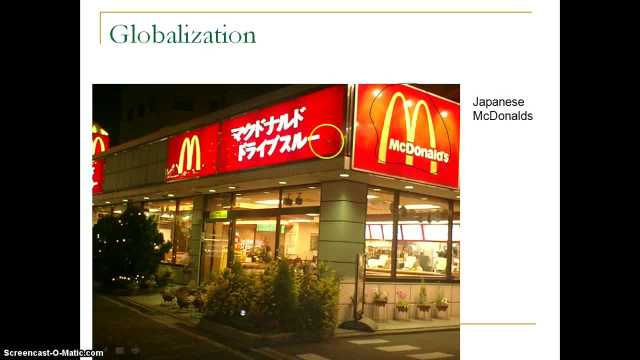 where it says McDonald's here over in the corner. But even if this was gone and you saw this giant M, this golden M, you would know that it was a McDonald's. and you may even see Ronald McDonald here hiding behind the bushes. But anyway, so you saw the giant golden arches M. 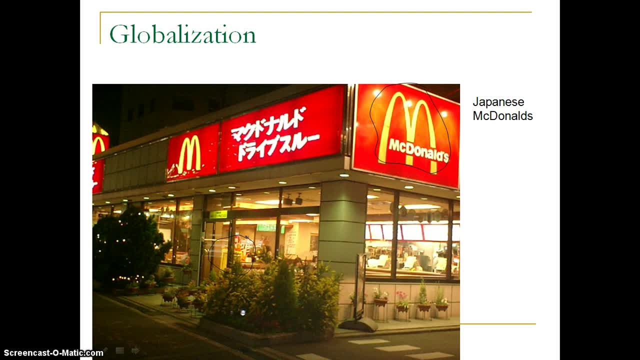 It looks like McDonald's had some problem here. You would know that was a McDonald's, and so that is an element of globalization, this international recognition of whether it's individuals or maybe a song, or maybe it's a brand or a company or whatever. 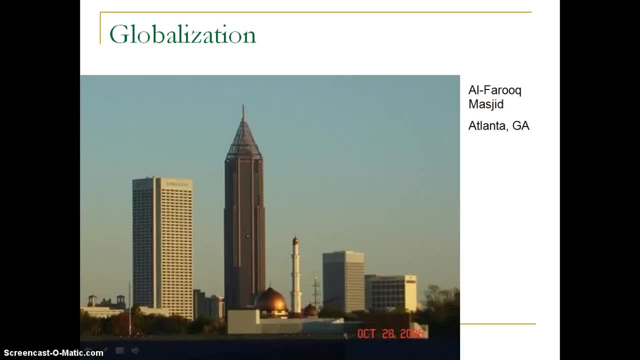 That is going to be fostered by globalization. Maybe we talk about not just the economic landscape, but also the cultural landscape as well. This is actually in downtown Atlanta. This picture was taken back in 2006.. This is a mosque that is built right in downtown Atlanta, right off of I-75.. 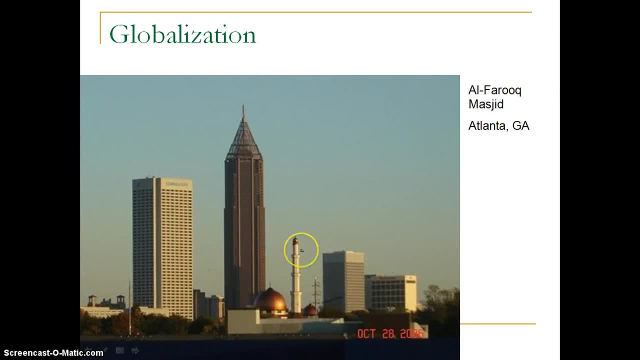 I've actually been there to visit. That's going to signify the changing cultural and of course this is dealing strictly with religious and of course with the religious, ethnic and other things. You see, the cultural landscape of a place like Atlanta, Georgia is changing. 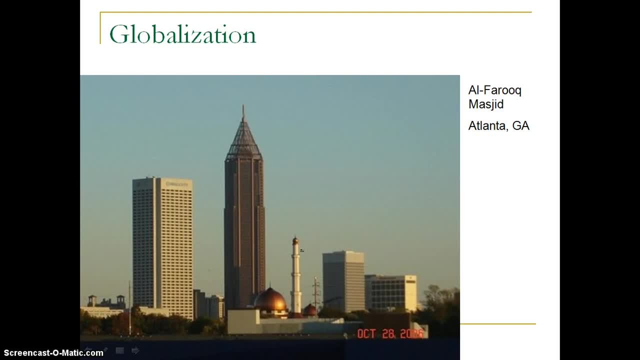 Of course, if the cultural landscape of Atlanta Georgia is changing, you know that the cultural landscape of Portland and, of course, if the cultural landscape of Atlanta Georgia is changing, you know that the cultural landscape of Atlanta Georgia is changing. 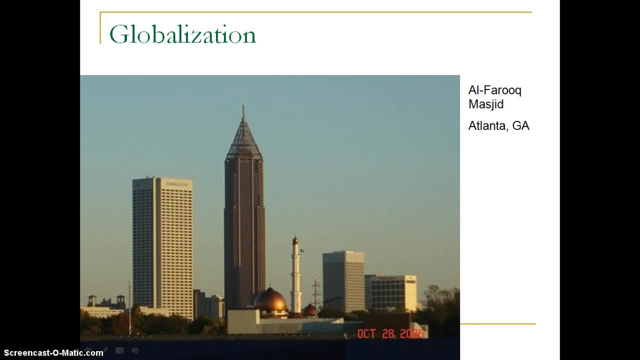 All over the world, especially in the United States with larger cities, is going to be changing. If there's a large enough Muslim population in the Atlanta and metro Atlanta area to warrant the building of a mosque, and a relatively large mosque at that, and so again that's going to be indicative of the changing population. 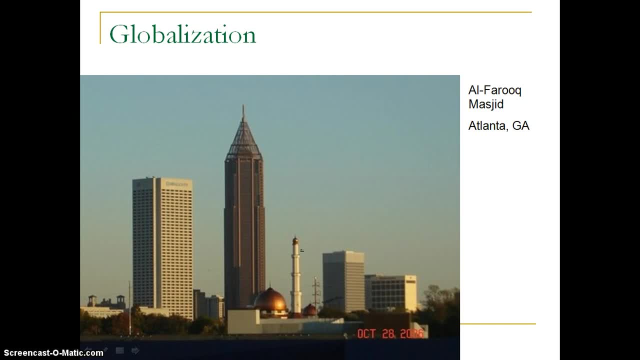 So you could talk about people moving across the world, whether it's for jobs or other things. But again, we're coming into contact with other types of people who come from different backgrounds and have different cultures, and so that's going to be indicative of the changing population. 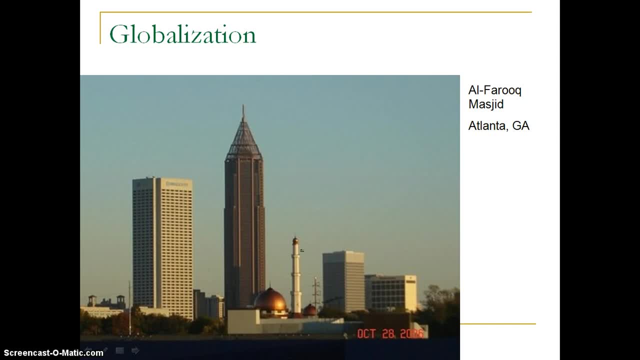 So again that's going to be indicative of the changing population. So again that's going to be indicative of the changing population. So again that's going to be indicative of the changing population. And so that's going to be changing the cultural and also the physical landscape. 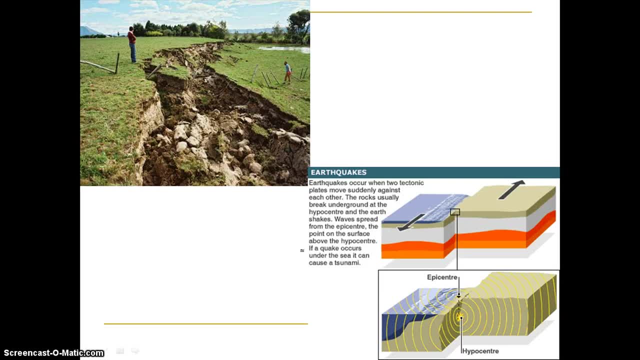 You could look at other things like earthquakes. This doesn't necessarily have to do with globalization, but we're talking about the way an area is impacted. You look at an earthquake and you can think about what exactly is the physical element that causes an earthquake to occur. 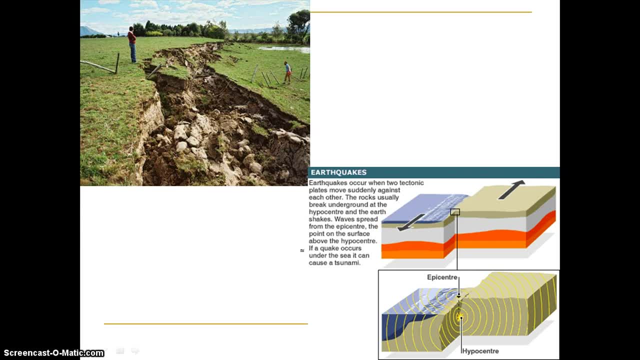 And then you also look at the way that that impacts not just the physical landscape but also the human landscape. Think about a place like San Francisco, California. Even though it has frequent earthquakes, we have a very large city that's located there. 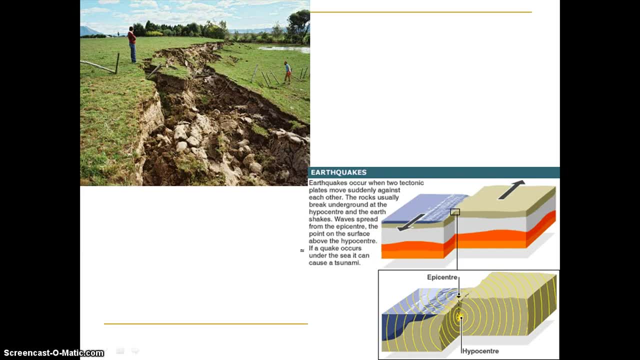 And so how is that going to impact the people? How is that going to impact the economy? How is that going to impact the infrastructure and the way that buildings are built, roads are built, How is that going to impact things like insurance and property values in terms of the cost of people living there? 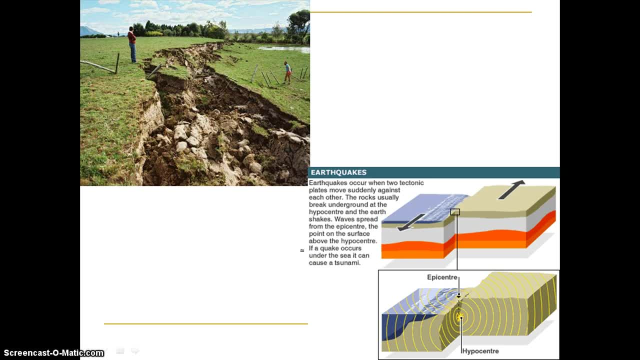 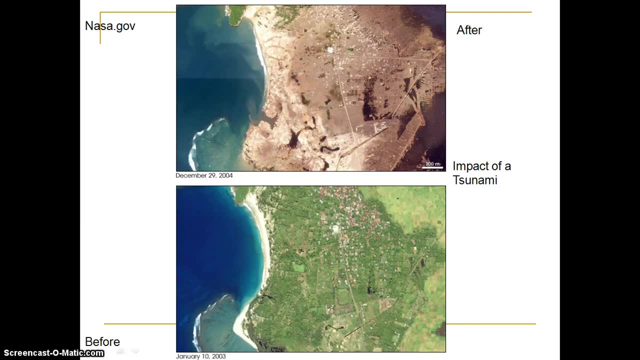 And so you really start to dig and you start to see how people have to live different types of lives based upon the physical environment, Or something like a storm Or a tsunami that is, that could, of course, devastate a particular area. So this was a tsunami that occurred in 2003.. 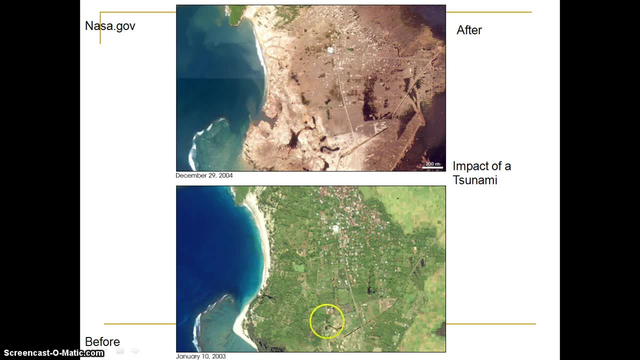 And these are a couple pictures taken from NASA's website, So of course you see the prior, the before picture And then you see the after picture here. So in the impact of the island there based upon the tsunami, And so you think about not only the impact that the tsunami had on the physical landscape, 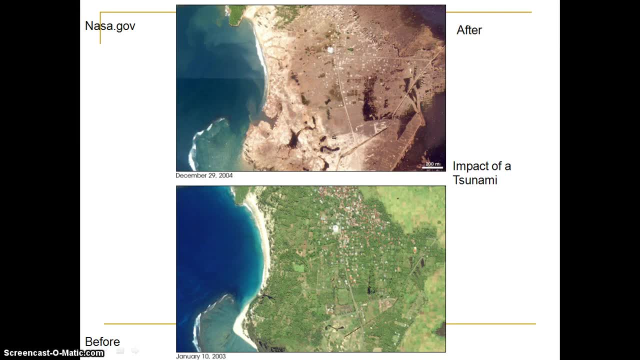 but also the people that are living there. Are the people able to come in? Are they able to come back to that location? Are they going to be dispersed? And then, if they are dispersed and go live somewhere else, then how is that going to impact the place where they've gone? 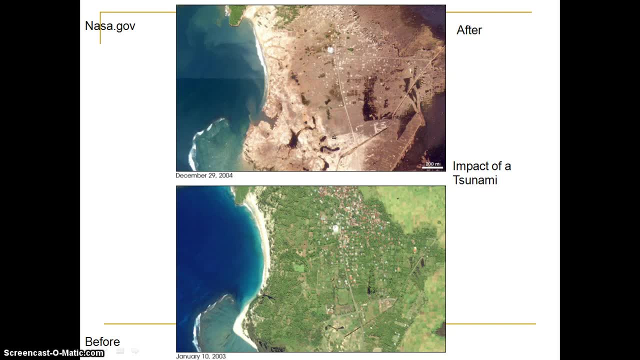 And so you talk about the movement and movement of people, taking their culture with them, Taking their, you know, their ideas with them, You know. and if people stay there, then how are they going to change their living, Whether it's maybe a certain, a different type of housing or protective barriers to keep the tsunami from having as much of an impact? 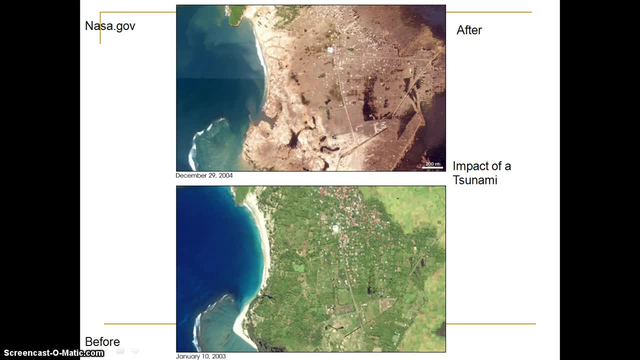 Have you ever been down to the coast of Florida, Or you've been to the really the coast coastal towns of any kind? you see a lot of houses on stilts And again, a lot of that has to do with, you know, weather that comes through and might cause the ocean to rise very high. 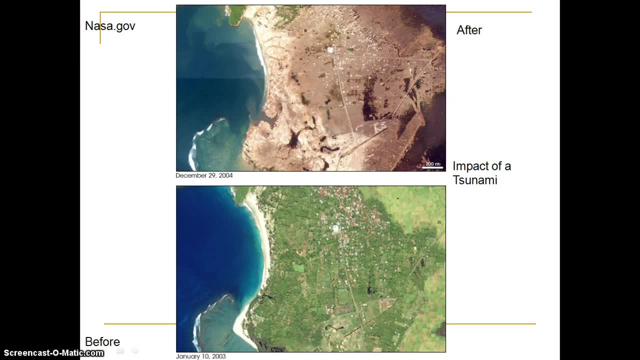 And so, instead of damaging the whole house, you have these houses on stilts that are going to allow the water to pass right under the house. Maybe it gets the car or whatever, but it's not going to destroy the entire house. And so those are some. those are some adjustments that people are going to make as they're living in an area and as they have to interact with the physical. 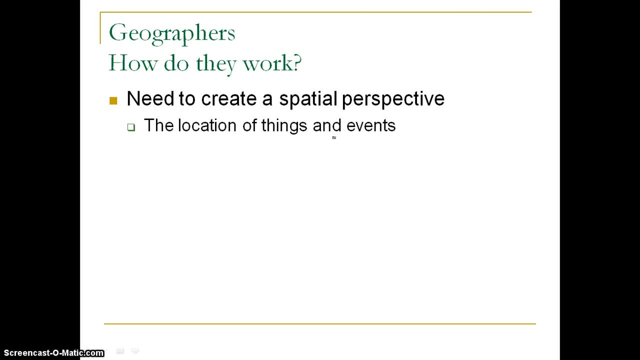 the physical environment. So when we look at geography and we begin to understand just the basic elements of geography, if we look at geographers and what it is that they do, let's talk for a second about how they work and what exactly it is that they're going to be doing. 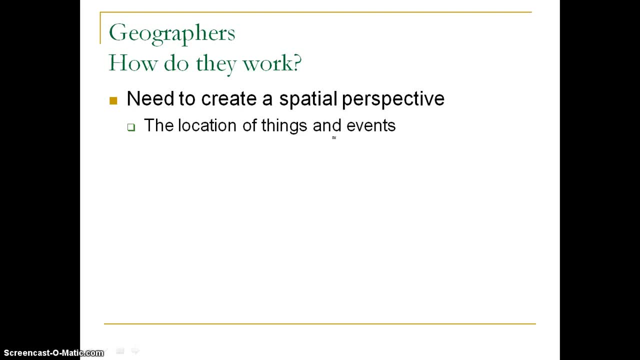 And we talked about space a little bit earlier. So the first thing that they're going to need to do is try to create a spatial perspective. So, again, it's not just the events that are going on, but you also want to look at where the events are. 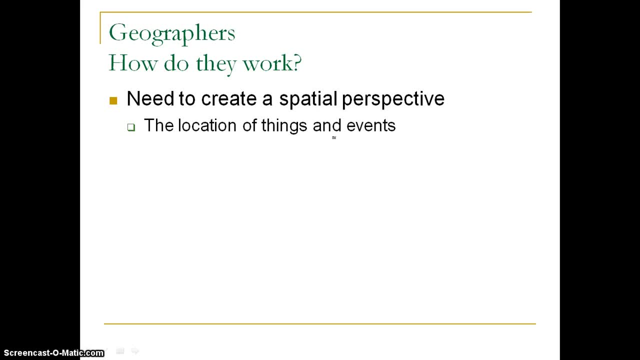 where certain events are And see if things can be tied together Again, whether it's a human event, whether it's an environmental event, and then not only where those things are, not only what's taking place, but also where those things are taking place. 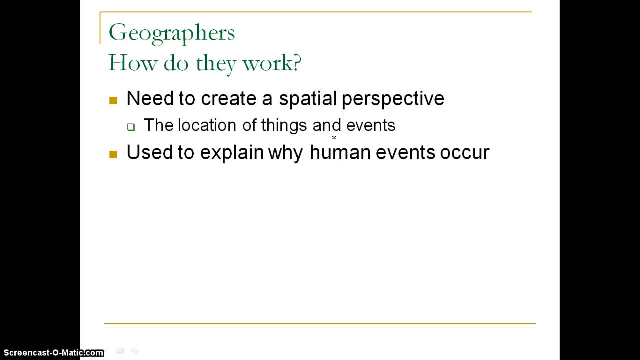 Okay, And then we want to explain why human events are going to occur in a specific location, And then we can take the different events that are occurring and we can try and tie those together and see how those different things, different things- might be related to one another. 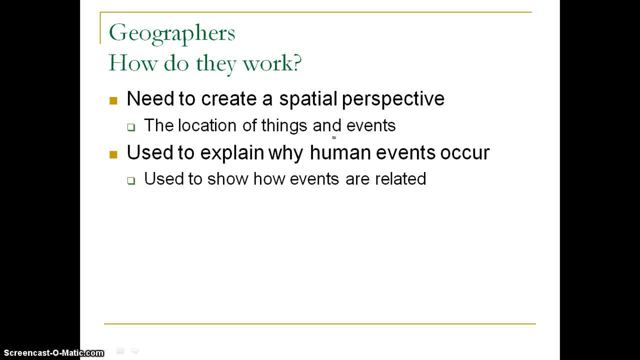 Now what we might find is that there is absolutely is no relationship between certain events, And they may be there as just an absolute coincidence, Okay, But if we look at some other, if we look at the events and we record them, we notice that they actually are related to each other. 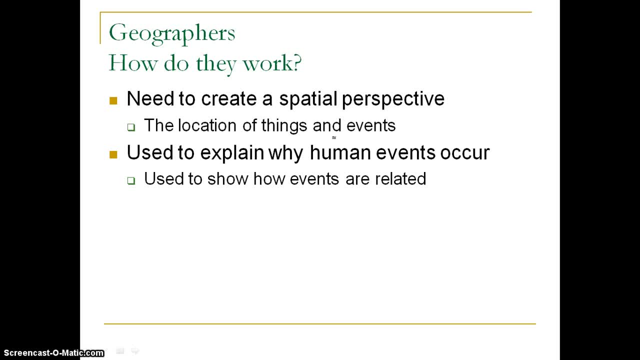 We can. we know that there is some sort of relationship that exists between either the people maybe that are living there or the people in their environment. It just depends, And so it really just takes some investigating and data collection, and that's what we'll talk about. talk about next. 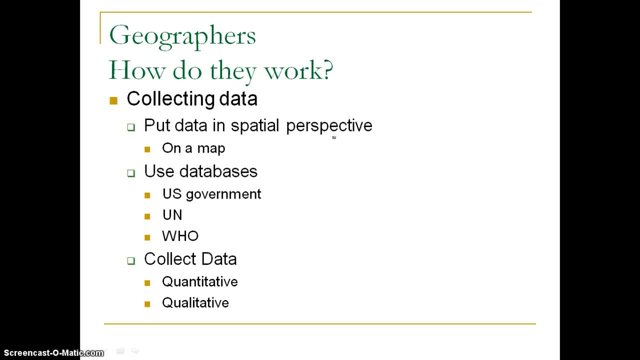 And so, when we talk about geographers and the work that they do, one of the most important elements that geographers are going to participate in is the collection of data, And this allows them to create that spatial perspective. So it's not just about the data collection itself, though. 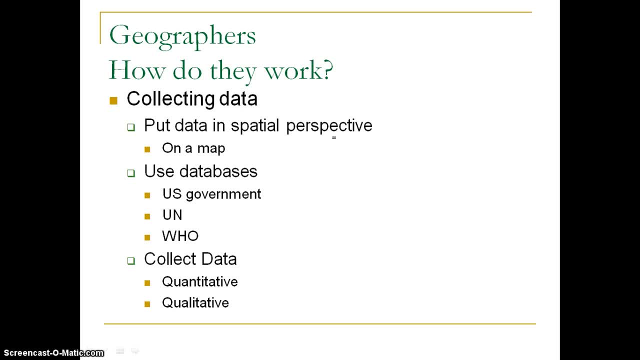 You actually have to take that data and you have to put it in spatial perspective. So that's why they're going to place their data On a map. And so when we look at the different types of maps- whether it's a choropleth or it's an isoline or it's a proportional symbol- 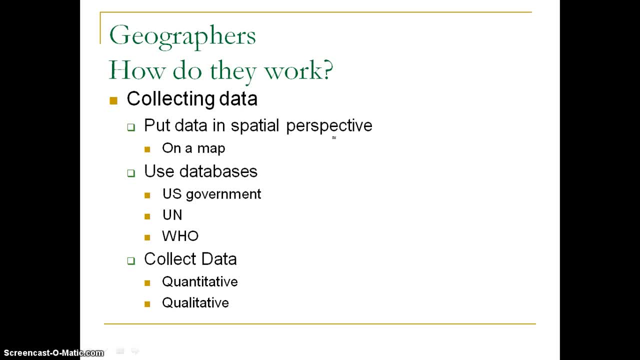 Those are the different ways that geographers are going to choose to display the data that they're collecting, And so that helps us to understand how that data is related to the space that it's taking place in, And so geographers can do a lot of different things. 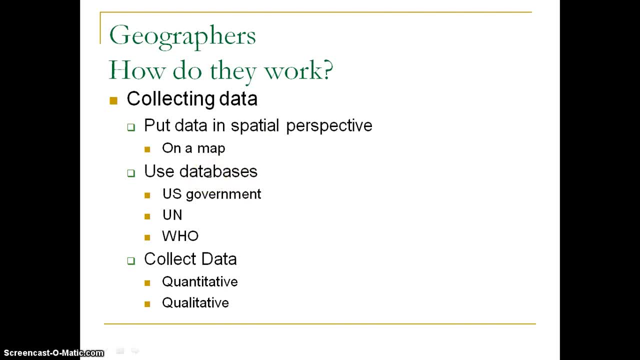 You know, one of the things they might do is use a database to collect their information and plug in So they can either look to different sources, Different types of governments- You know you have the US government you can go to to collect data. 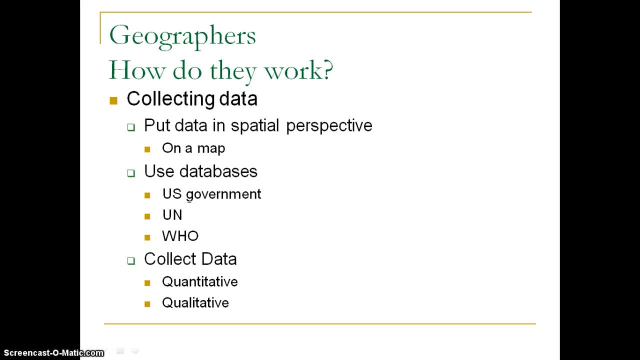 You look at like the US Census Bureau, You maybe can go to the CIA World Factbook- A lot of other different databases that are there. You can go to the United Nations and look at some of their databases they have, maybe on population. 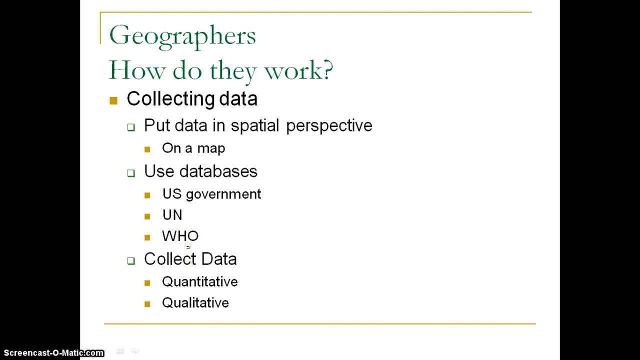 And then maybe even something like the World Health Organization. There are a lot of others. These are just some basic examples And there are a lot of other independent databases. You might go to Gapminder, developed by Dr Hans Rosling, And he has a lot of information on population, on economics, on age. 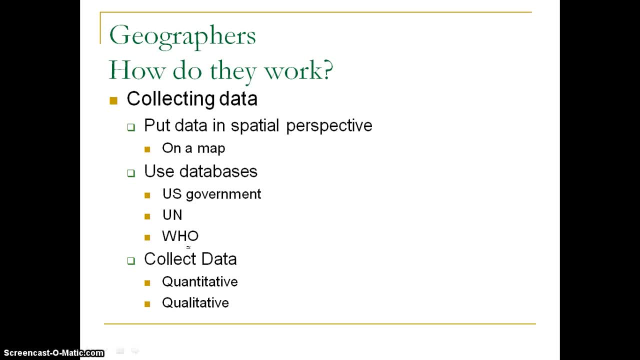 I mean, of course, age is related to population. So there's a lot of information and data collected on population that you can go in there and you could collect and then use that as a part of the data collection And so once the data is collected, you know again, you're going to put that on a map. 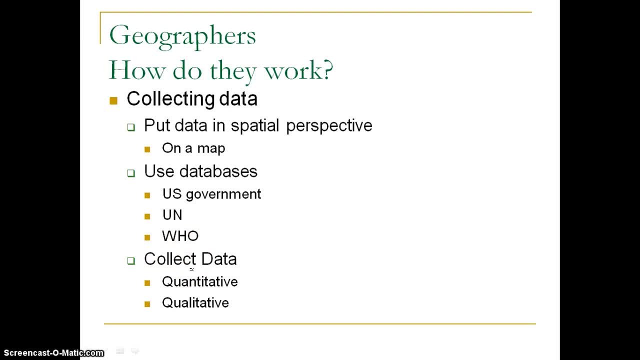 Now there are different types of data that can be collected, And I've talked to several geographers that do different types of data. You can either have what's called quantitative data or qualitative data. So the quantitative data is going to be hard numbers. 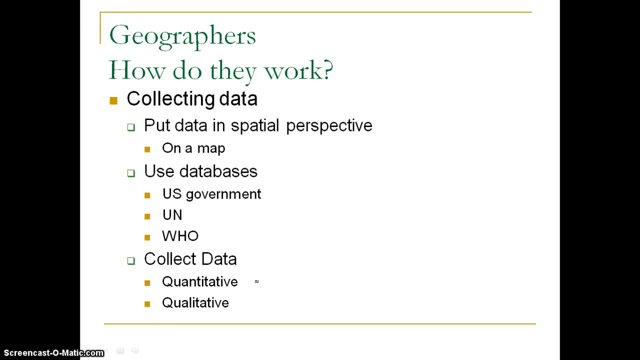 It's going to be, you know, actual counting of things and then plugging that into the map. Then you might also have what's called qualitative data. Now, this qualitative data is more interviews: talking to people, getting their perceptions and their ideas. 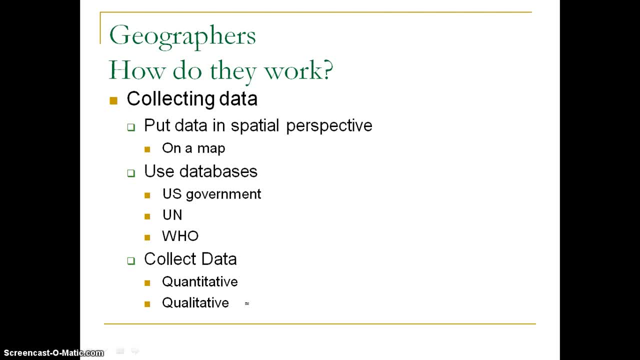 And then taking that data and then trying to translate it and make some try to make some sense out of it, And so these are a little bit different in terms of the world. It's not exactly what kind of data it is that they represent. 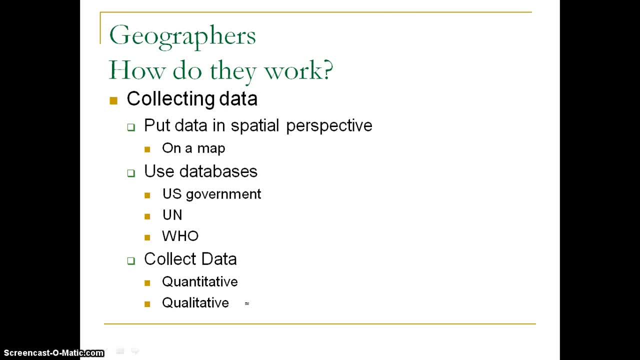 And so the geographers go through this effort of collecting the data so that they can then put that on the map- And we're not too map chet, so we'll get to that in just a little bit. But again, the most important thing that we can understand here is how the geographers are going to work to put things in a spatial perspective. 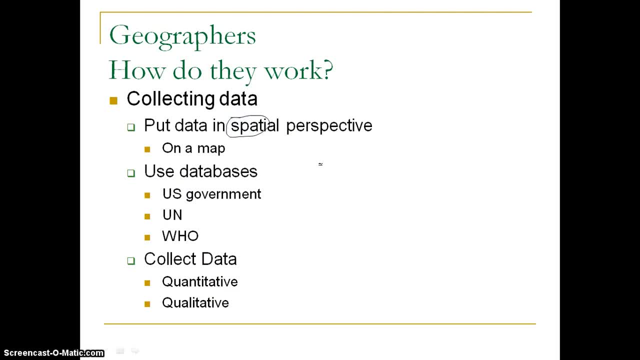 And, again, that's why we're going to be using, that's why they're going to be using- those maps in order to do that. So this is it for our introduction to geography. Our next video is going to be looking at the five themes of geography. 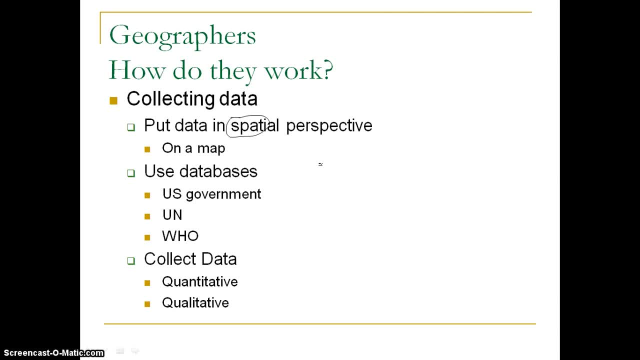 And so looking at what are some of the basic sets of information that we'll be looking at as we go throughout the year,